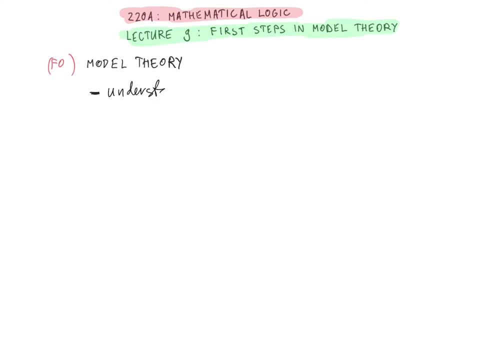 First, understand and develop methods to build models of a given first-order theory. Second, we try to actually classify first-order theories. So what is the concept of concept of concepts in the first-order theory? What do you mean, Hung? The concept of concepts is a fundamental concept of whatever is defined by an algebraic model. 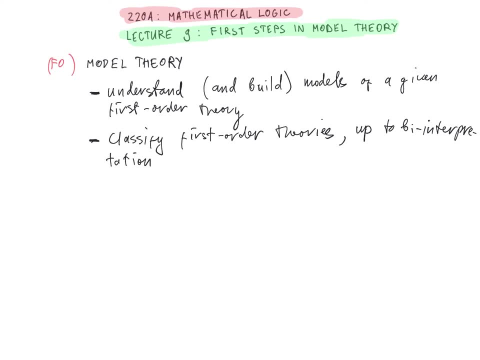 It reflects the complexity of a set of chemical components or the complexity of a set of things defined by a given first-order, And it reflects the complexity of the set of components of a given first-order theory. In other words, it's built on the idea of all the possible sets of components of a given first-order theory. 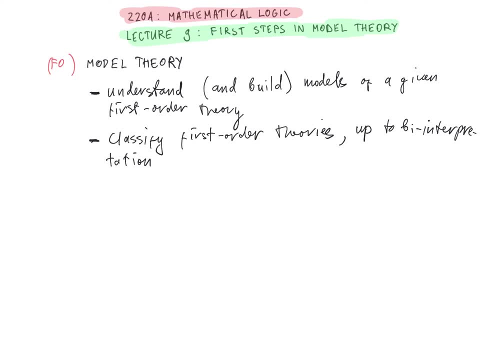 The project of classifying all first-order theories up to by interpretation, as we will see, is, of course, not plausible in any obvious sense, because there are just too many first-order theories and they can express all of mathematics So, more realistically, what this reduces to is to isolate interesting and useful. 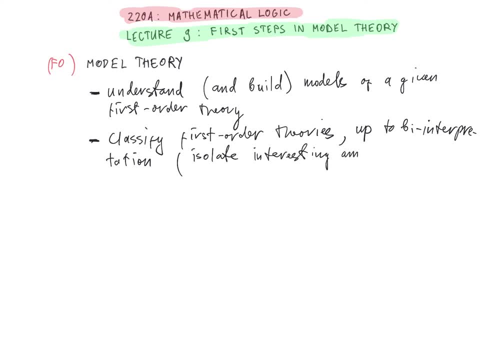 invariants of first-order theories which allow us to distinguish tame behavior from the wild one, or Godelian behavior, and we will see some examples of such dividing clients which allows to distinguish between the two, for example, stability. This is the one which will appear in this course. 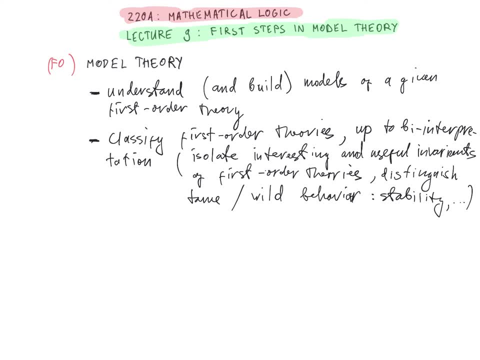 When we start talking about countable categorical theories. and the third line, which nevertheless is closely connected to the first two, is to understand And definable sets in models of a given first order theory. So, as we will see, all these three kinds of questions are closely connected and inform. 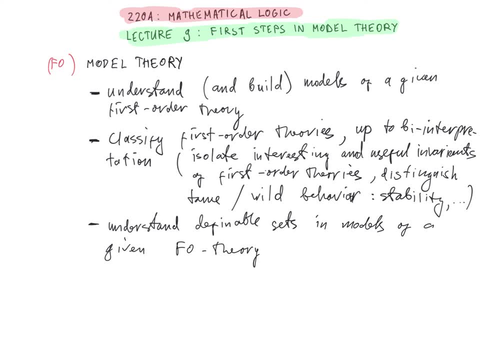 each other In terms of more concrete results. for the first question- understanding and building models of first order theories- some specific results that we will consider are going to be the Loewenheim-Scholem theorem, which allows us to build models of a given theory. 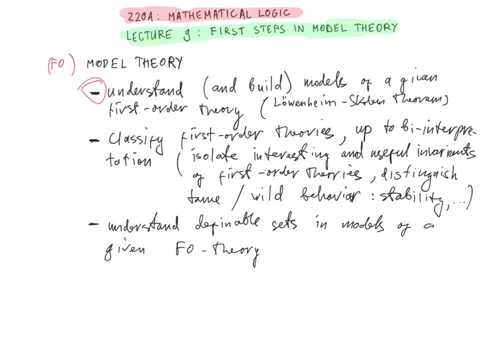 of different sizes, And we will also talk about saturated models. These are somehow rich models in which a lot of things that can happen already happen, And we will also talk about prime models etc. So we will study various special kinds of models of a given theory and methods of building. 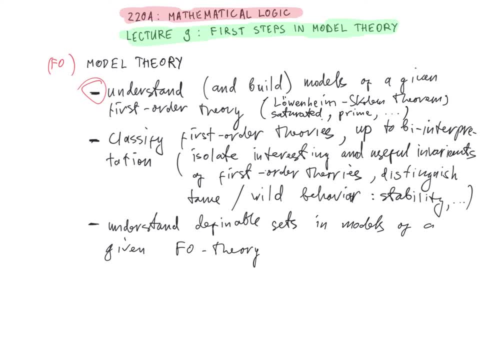 them. For the second part, we will discuss the notion of interpretation. so we will make precise this idea of coding one theory in the other And we will discuss various inversions: Invariance that allows to separate the wild behavior from the tame one. 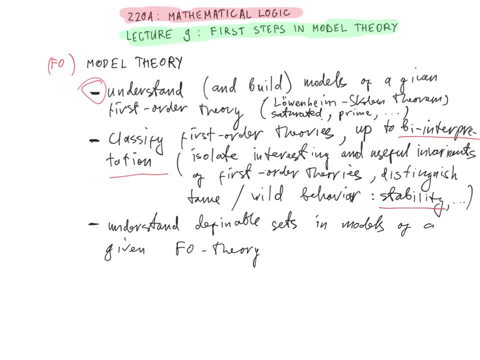 So, as I already mentioned, an important notion here will be that of stability, or kappa-stability for a given cardinal kappa. This will involve studying type spaces, certain stone spaces, compact Hausdorff dimension zero or absolutely disconnected topological spaces which are associated to a certain 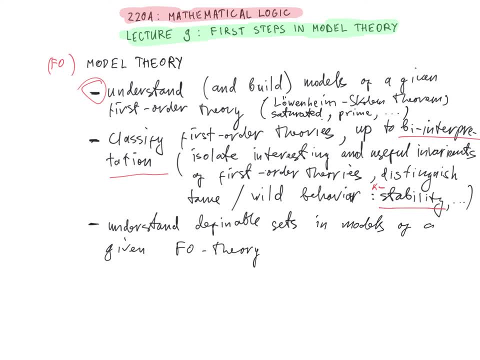 shape The Boolean algebra of definable sets of a given theory. So we will define all of those words. And for the last item, we will in particular discuss the notion of quantifier, elimination, Model, completeness And some other notions Which allow to express that definable sets in a given theory take simple or understandable. 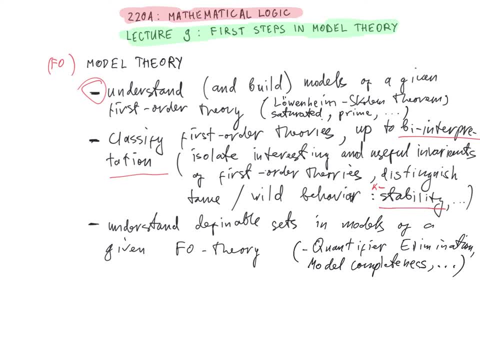 form which can be expressed already by formulas without quantifiers, in the first case, or by formulas with only existential quantifiers, in the second case, etc. And we will consider some particular examples in which these methods apply. So this is a quick summary of some of the topics we will discuss. 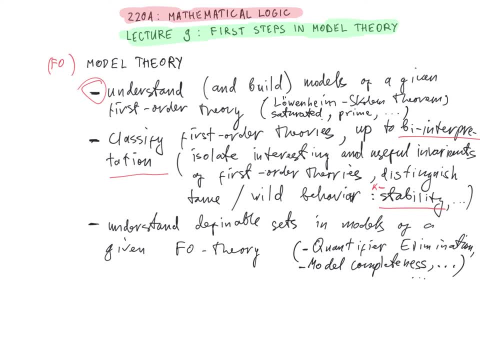 And if you have any questions, please feel free to ask them in the comments. Thank you, In all of these topics we will deepen the connections between syntax and semantics, where the first fundamental result was Gödel's Completeness Theorem, and we will see various 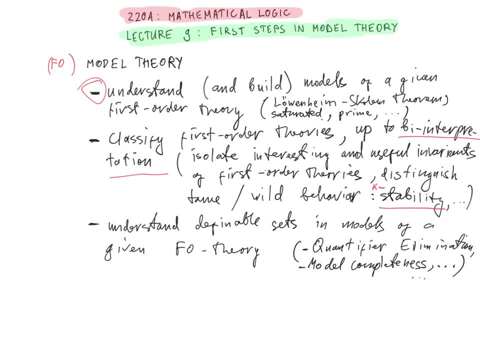 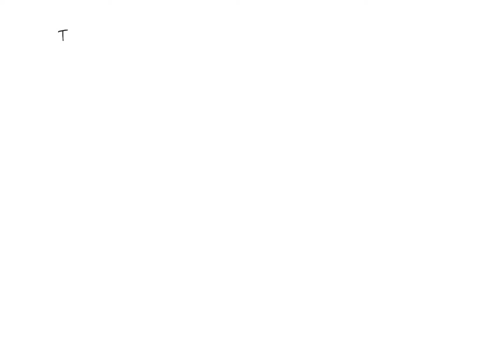 deeper connections, which allows to establish correspondence between certain syntactic properties and their semantic counterparts. Let us begin discussing some of the simple initial results and notions to set up the terminology that is used in model theory. So first of all we state the very important compactness theorem of first-order logic. 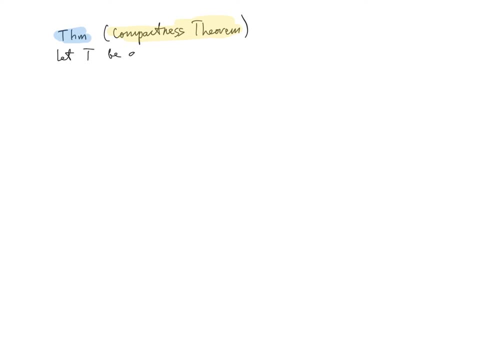 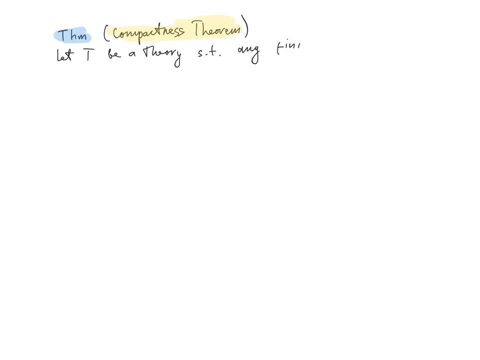 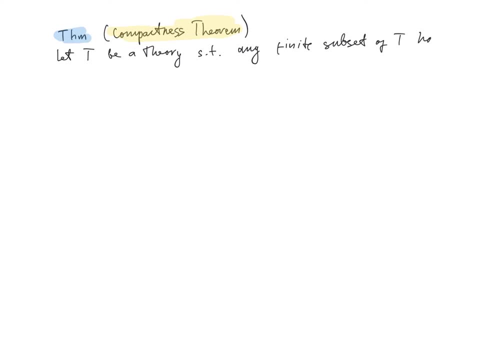 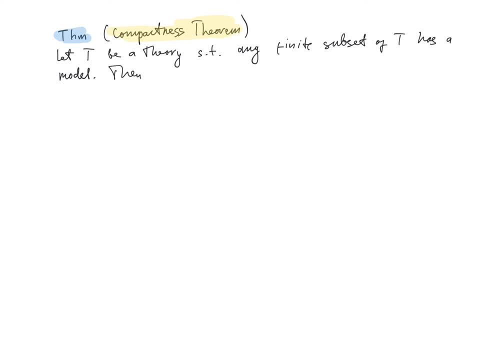 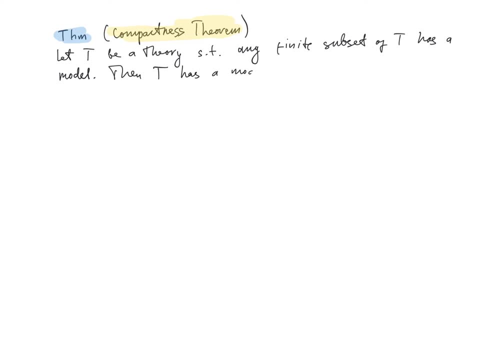 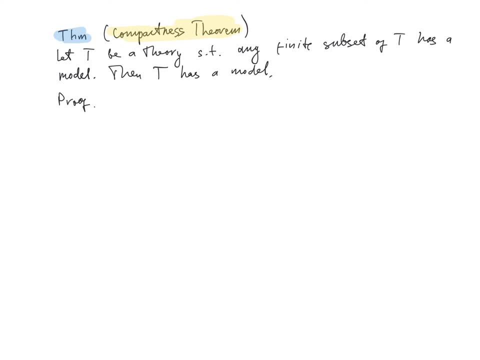 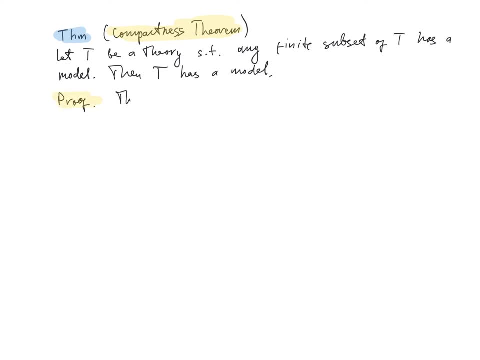 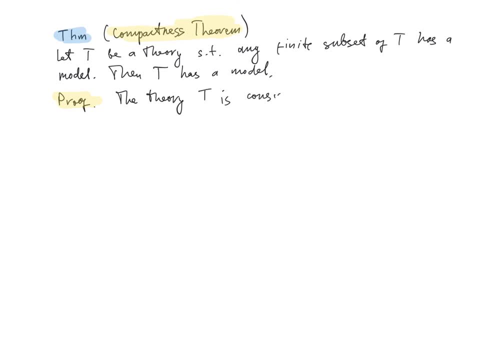 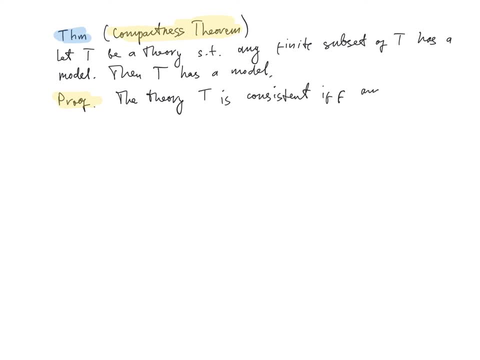 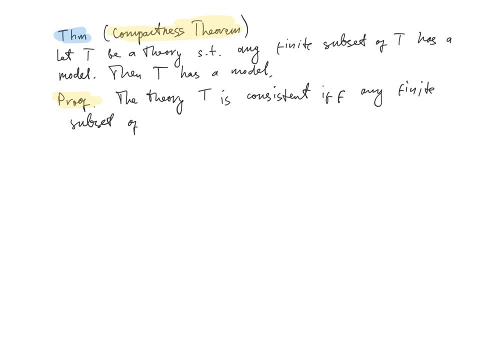 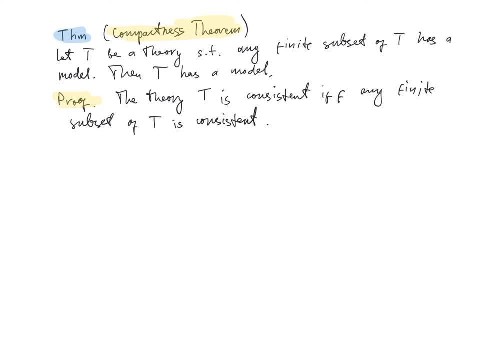 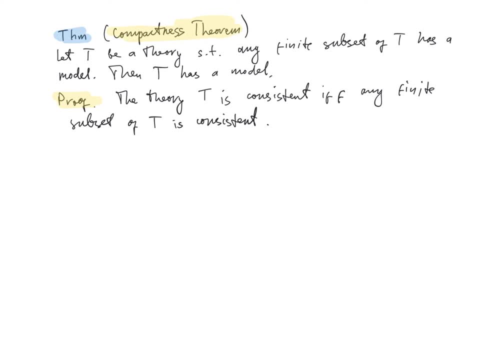 both phi and not phi in the sense of the existence of a formal proof. now, of course, we have this equivalence simply because any proof can only involve finitely many sentences from the theory t, so we just have to take the finite subset containing all of the sentences that appear. 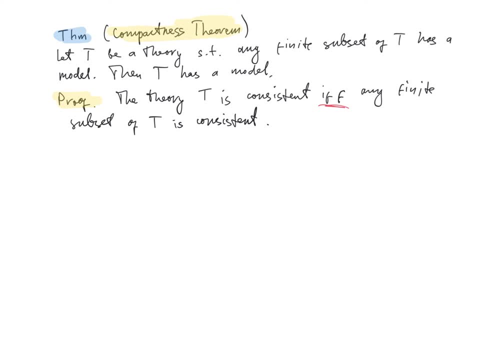 in the proof of phi and in the proof of not phi for some first order sentence, phi in the case t was inconsistent. this would give us a finite inconsistent subset of t already. but also by the completeness theorem we know that a theory has a model if, and only if. 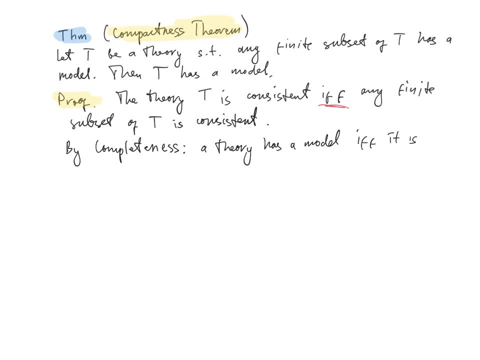 it is consistent. so now, combining these two claims, we see that a theory has a model if, and only if, every finite subset of this theory has a model. here we have obtained the compactness theorem as a simple corollary of the completeness theorem proved earlier, and now this: 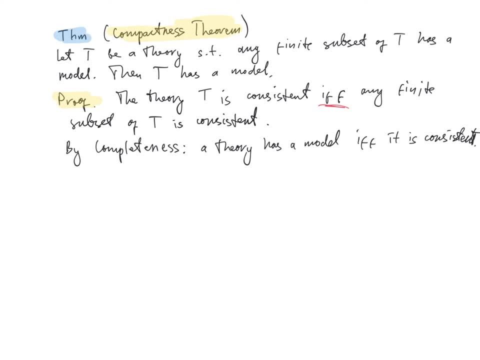 As a result, the compactness theorem is originally due to Gödel in the case of countable languages, and due to Maltsev in the case of languages of arbitrary cardinalities. From the point of view of model theory, this consequence of the completeness result for 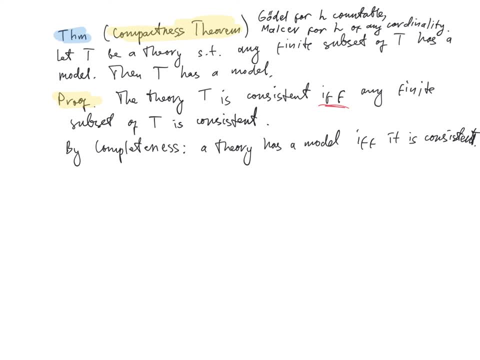 first-order logic is probably the most important result, first of all because it only talks about semantics. it only talks about the existence of models and doesn't discuss formal proofs. As we will see later, when we start talking about ultra-products and ultra-filters, we 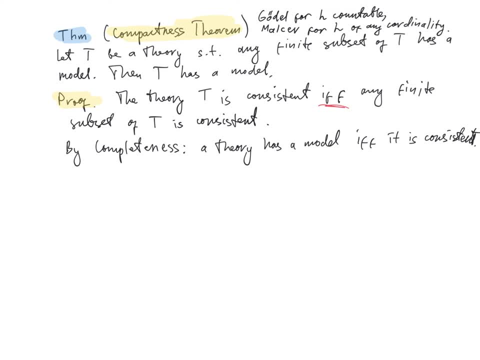 will see that there are also proofs of the compactness theorem, which can also be done fully semantically and avoid using the completeness theorem. so we will see a proof like that later in the course when we start talking about types. But let me just remark for now that compactness here actually will correspond to compactness. 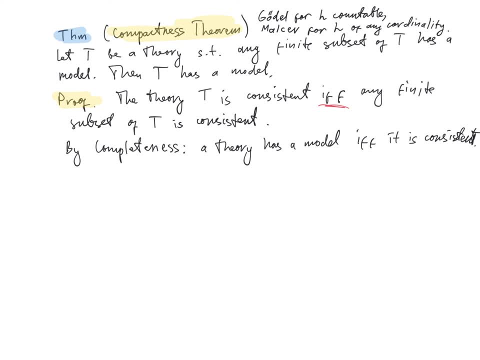 in the sense of topology, of a certain topological space associated with a certain compactness. So we'll return to this topic later on. Okay, so for now let us set up some notation definition. let M and N be two L-structures. 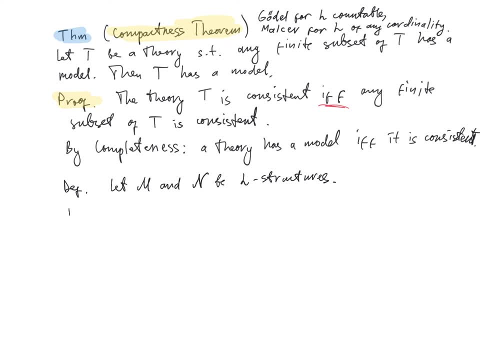 in some given first-order language E. We are interested in the situations when both structures satisfy the same L-sentences. so we will say that these two structures, M and N, are elementarily equivalent, denoted as M is equivalent to N if they satisfy the same L sentences. 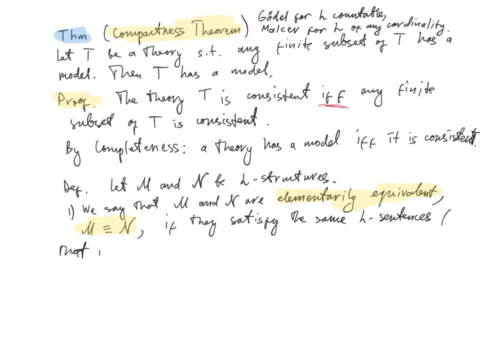 In other words, if the complete theory of M is equal to the complete theory of N. next we define the notion of substructure. So assume that M is a substructure Subset of N, where M- N are the base sets of the corresponding structures, M- N respectively. 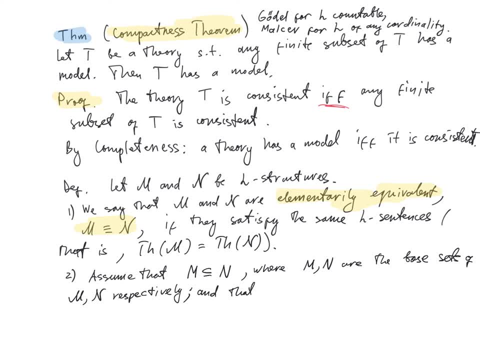 And also that we have, for every Subset of N, where M- N are the base sets of the corresponding structures, M- N respectively. And also that we have, for every Constant C, a constant symbol from the language L that the interpretation of this constant. 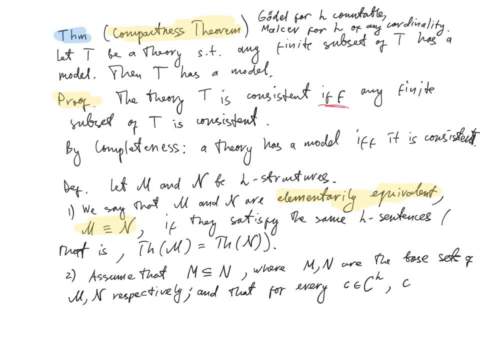 symbol in the structure N is equal to the interpretation in the structure N. So in particular the interpretation of this constant symbol in N is an element of the base set M, That second. we also have that for every relation symbol r of a given r-ity. 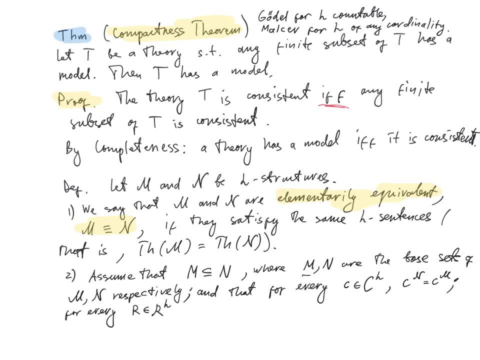 and in the language L, the interpretation of the symbol in the smaller structure M, is given by the restriction of the corresponding interpretation in N, restricted to the set M, to the power N. so the interpretation in M is just the restriction of the interpretation in N to the base set of M. 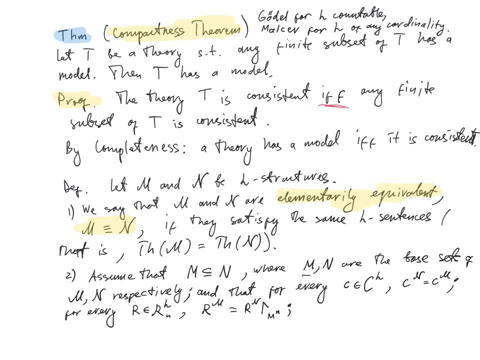 and finally assume that also for every function symbol f in the language L of r-ity N we have that this interpretation of this function in M is obtained by looking at the interpretation of this function symbol in the bigger structure N and again restricting it to the base set M to the corresponding power N. 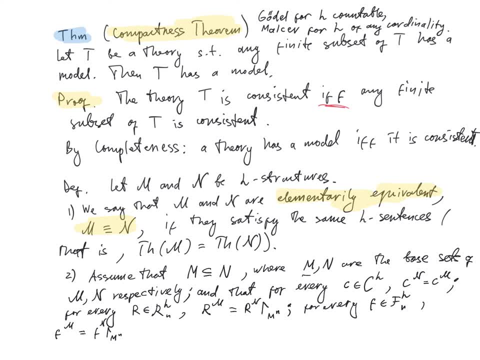 so, in particular, it follows that this underlying set M is closed under the function, given the interpretation of this symbol. so if all of these three conditions hold, then we will say that M is a substructure of the structure N, which is denoted. 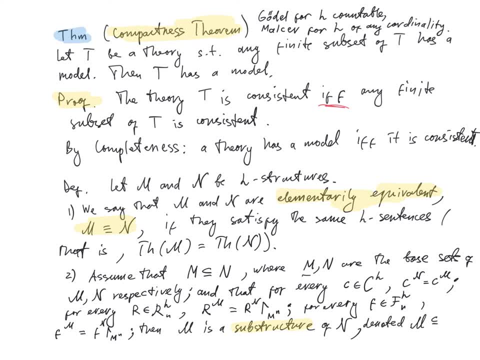 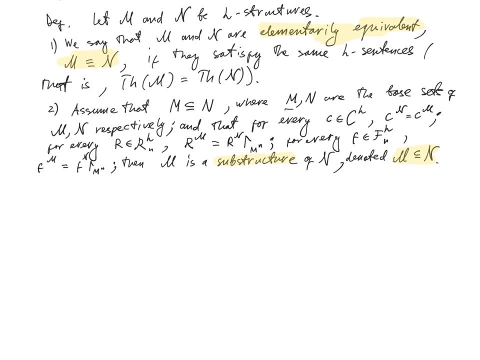 by writing that M is a substructure of N. Now we define a stronger way in which a structure can sit inside the other structure by combining 1 and 2, so we have 3,. assume that M is a substructure of N. 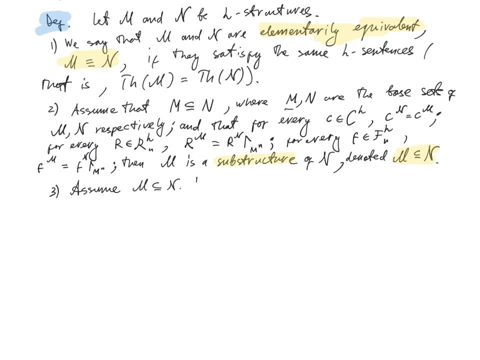 and then then we say that M is an elementary substructure of N, and in this case N is called N elementary extension of M, if for every L-formula phi of X1 through Xn, so all of the free variables. 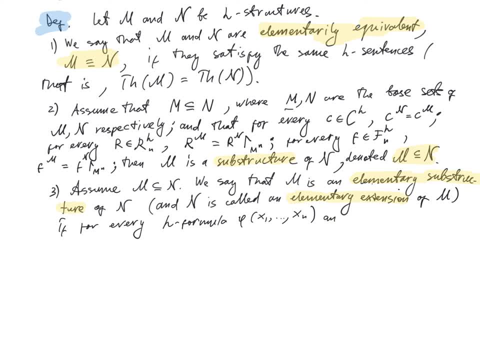 of phi are among X1 through Xn and every tuple a bar of length n, so consisting of some elements, a1 through an, from the corresponding power of the base set of the smaller structure, M. We have that M satisfies phi on this tuple of elements a bar if, and only if, n satisfies phi on a bar. 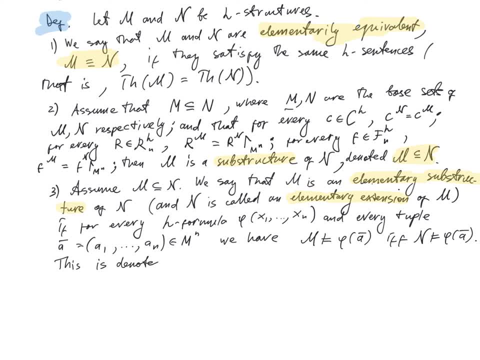 And this is denoted by M an elementary substructure of n. Okay, Thank you, Thank you. Thank you. We will also write that M is a proper elementary substructure of n. so the strict inequality symbol if M is an elementary substructure of n and the base set of M is strictly smaller. 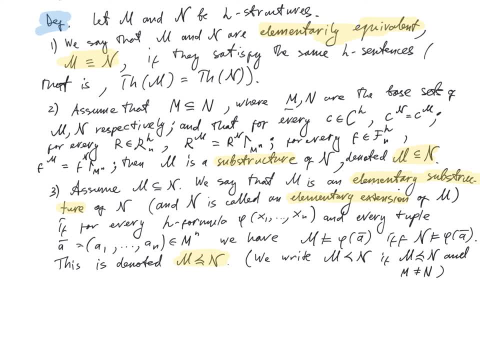 than the base set of n. So there are some new elements in the base set of n. First we have that if M is an elementary substructure of n, then also M is elementarily equivalent to n. This holds by applying the definition of elementary substructure to formulas with zero variables. 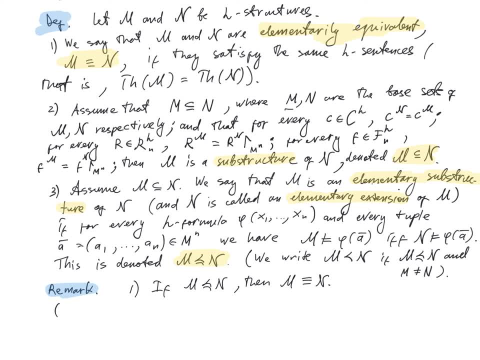 hence to L sentences. Okay, So because, in particular, if M is an elementary substructure of n, then in particular we have that for every sentence, phi, ie formula without any free variables. we have that M, M satisfies phi if, and only if, n satisfies phi, on the empty tuple from the base set of 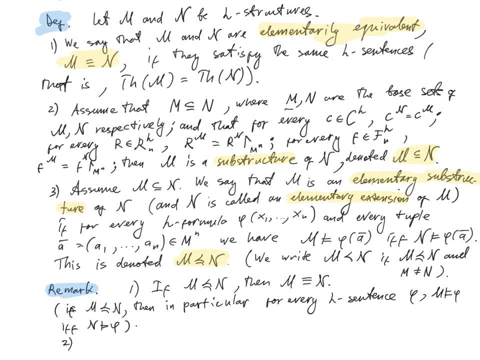 M. So this is part one And part two. if the structure M is isomorphic to the structure n, then the elementary substructure of n is strictly smaller than the base set of n. then they are also elementarily equivalent. More precisely, we can show that if F is an isomorphism from M to n, which remember- 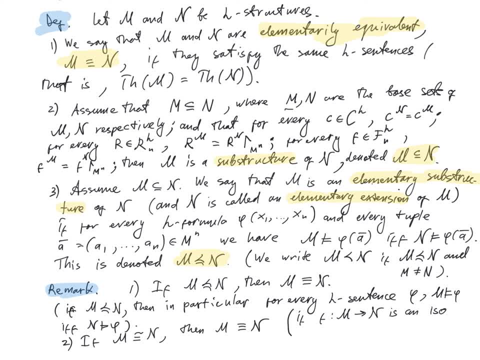 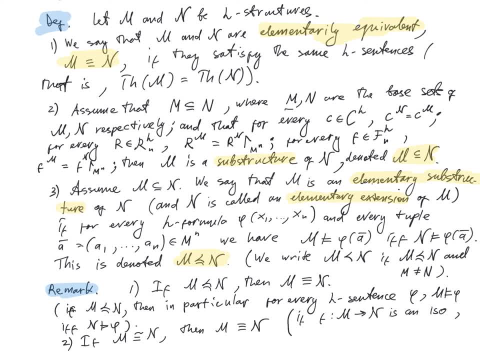 Okay, So given a structure that is an isomorphism, we can check by induction on the height of a formula, phi, that if M satisfies phi on the given tuple of elements a1 through an from the base set of the structure M, then this happens if, and only if, N satisfies phi on the 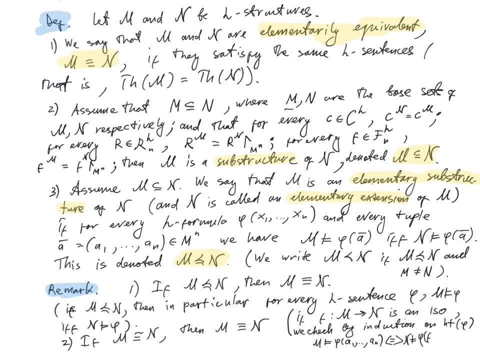 tuple of elements that F maps the AIs to. So phi of F of a1 through F of an holds. Now the definition of isomorphism, of F being an isomorphism, guarantees that this happens for all formulas of height 0, and then we can argue inductively the 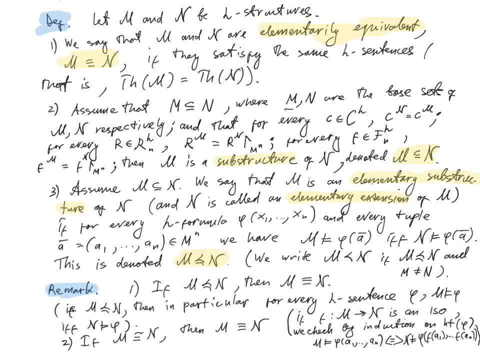 only non-trivial case has been adding a quantifier. but in this case if some formula is satisfied, some existential formula is satisfied, for example in M witnessed by an element- then we can look at the image of that element in N by applying F to it and we will see that the corresponding 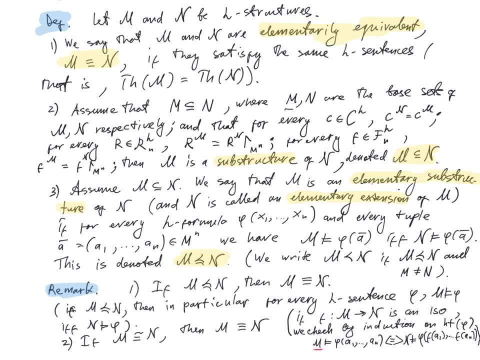 element F of a is going to be a witness for the satisfaction of the same existential formula in the structure M. So simple inductive argument shows that the isomorphism of M and N implies the elementary equivalence. However, we will see that the converse is not true in general, that for any 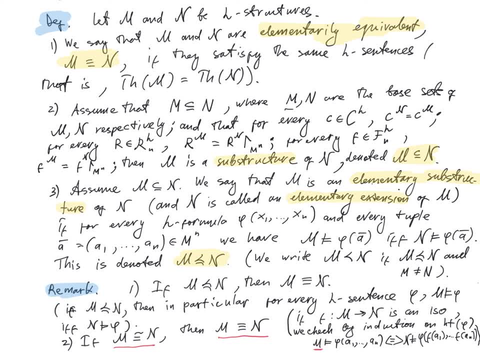 infinite structures M and N. the notion of elementary equivalence is much weaker than the notion of isomorphism, So we'll see many examples of it. In particular, elementary equivalence cannot distinguish the cardinality of the base set of a structure as long as it is infinite. 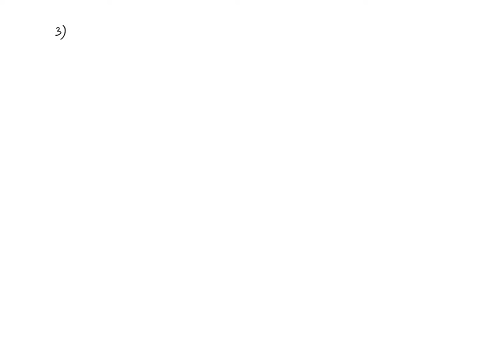 And the third part of the remark. we stress that if M is a substructure of N and M is elementarily equivalent to N, this does not imply in general that M is an elementary substructure of N. So of course, if M is an elementary, 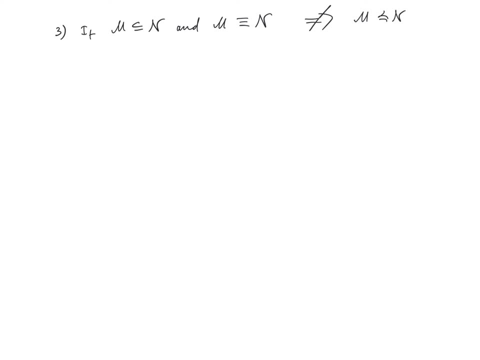 substructure of N. by part one, we see that M is a substructure of N which is elementarily equivalent to N. so this implication does hold. However, the converse implication doesn't. Let's consider an example which illustrates this. So consider: 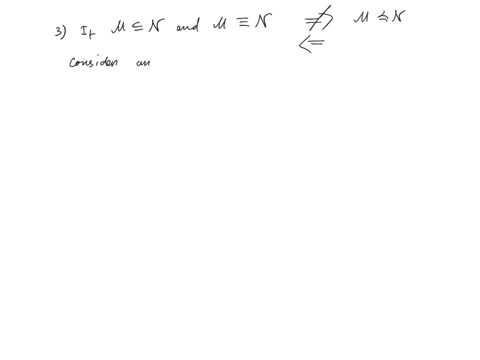 a structure in the language of linear orders. Let's take n to be the set of the natural numbers, n, with the usual linear ordering on it. and let m be another alert structure which we take to be the set of all natural numbers greater or equal than 1, so we are meeting 0, but again with the same natural 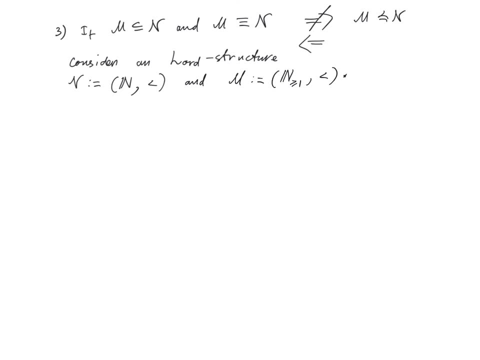 ordering induced from the natural numbers. So then we have- So these are two alert structures, of course, And we have that m. M is a substructure of n, since the ordering is the same, m just has a smaller base set. 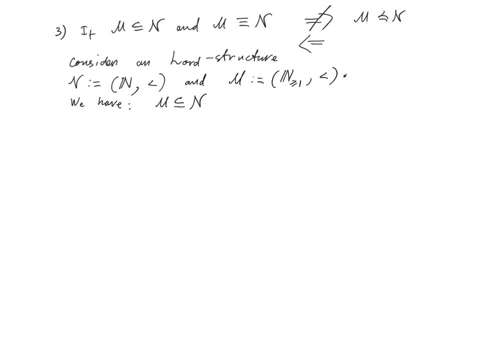 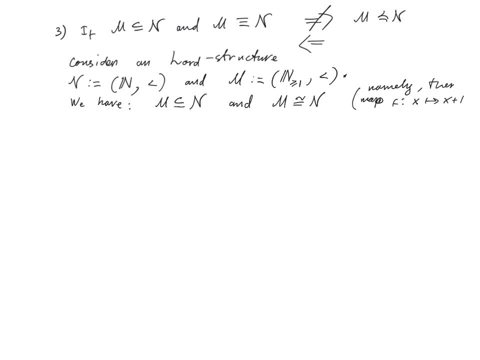 X to X plus one Is an isomorphism From the structure m To the structure n, since we only care about this map preserving the order, the only non-logical symbol in the language, it is clearly order preserving and gives some objection to the. 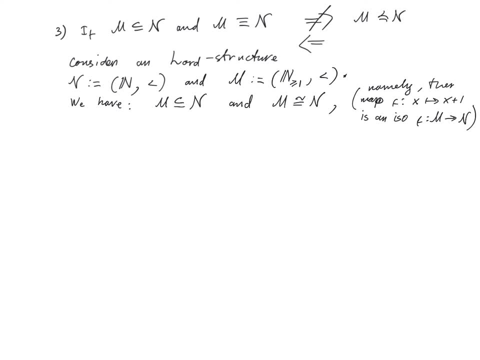 corresponding base sets. So these structures are isomorphic. so in particular we have that m is elementarily equivalent to n by the second claim of the remark, but on the other hand we have that the extension m is not elementary. To see this, consider an old formula phi in a single variable x. 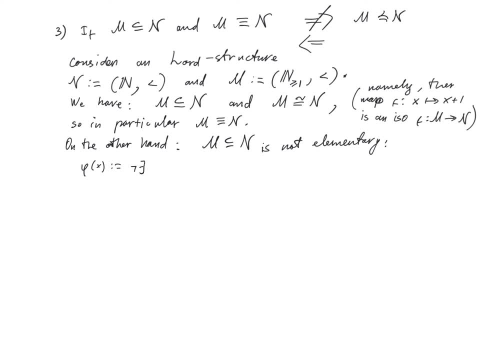 which says that there does not exist y, such that y is strictly less than x. so then we have that m satisfies phi of 1, so we take this 1 as an element of the base set of m, and there is nothing below it in m. so phi of 1 holds in m, but of course in n. 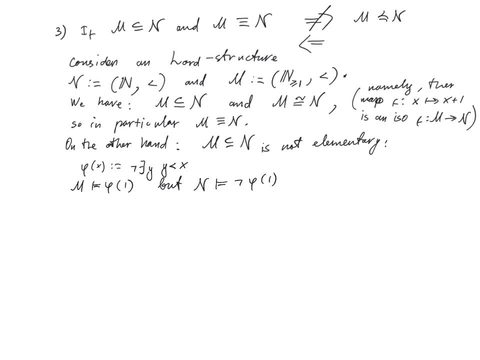 the negation of phi is satisfied by 1, because it has an element 0 which is below 1 in the ordering. So this example tells us that being a substructure and elementarily equivalent is not sufficient to be in an elementary substructure. 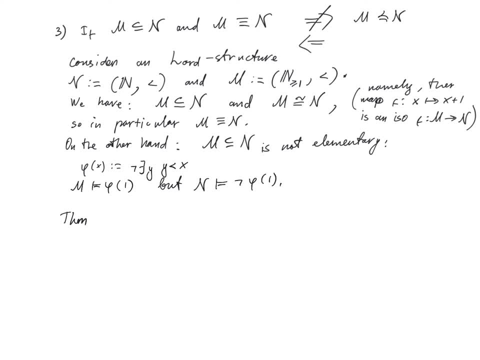 The next result provides a sufficient condition for being an elementary substructure. This is the so-called Tarski-Wott test for being an elementary substructure. So let m and n be two L-structures, so that m is a substructure of n. 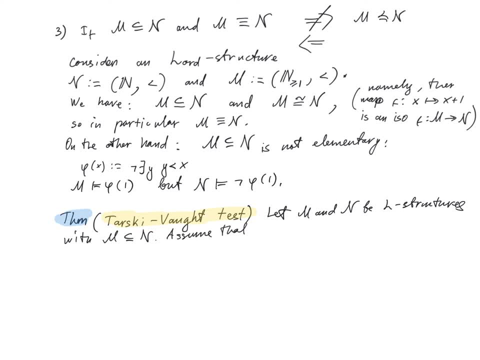 and assume that for any L-formula phi of x0 through xn and any tuple a-bar of length n, so consisting of a1 through an, so the length is one less than the number of the three variables in phi. so any such tuple a-bar from the base set of the smaller structure m. 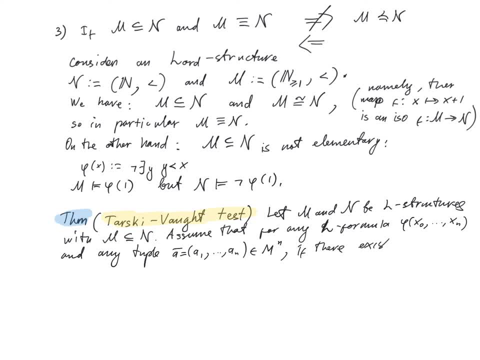 if there exists some b0, an element of the bigger structure n, such that this bigger structure n satisfies phi of b0 a-bar, then there exists an element a0 in the base set of the bigger structure n and the smaller structure n satisfies phi of a0 a-bar. 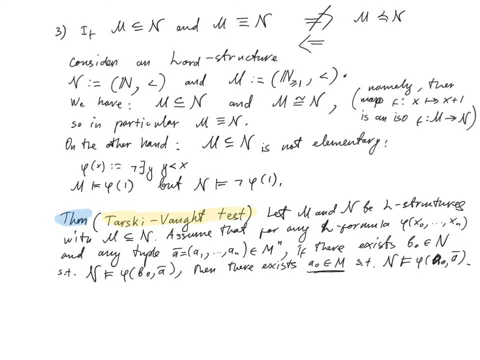 So assume that this happens for all formulas and all tuples a-bar of the smaller structure. whenever a formula satisfies a bigger structure, then there is already an element in the smaller structure witnessing a smaller structure. witnessing this, then we have that m is an elementary substructure of n. 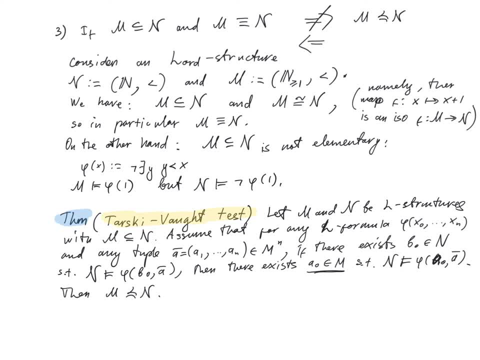 So of course, if m is an elementary substructure of n, then this condition would hold by the definition of elementary substructure. And the point is to show that this question reduces just to having this existential witnesses. So if a formula with parameters from the smaller structure is realized by something, 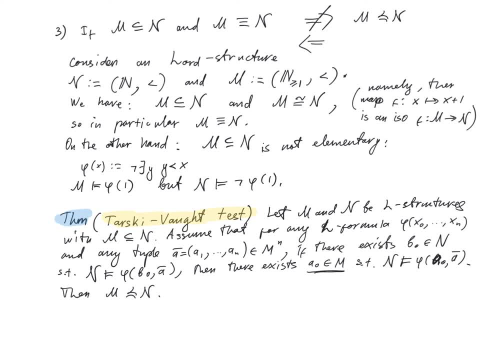 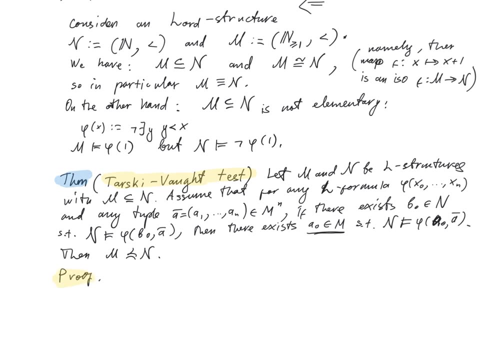 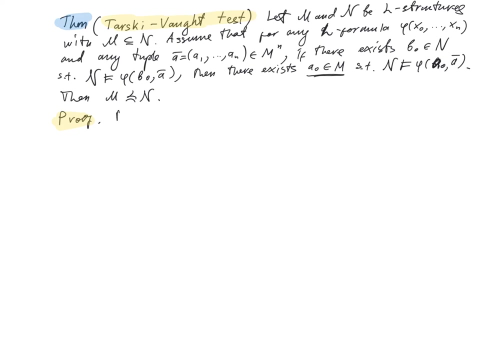 in the bigger structure, then it is already realized by something in the smaller structure as well. Let us prove that indeed Tarski-Watt test is a sufficient criterion for being an elementary substructure Proof. will show by induction on the height of a formula phi of x1 through xn in an arbitrary finite number of variables. 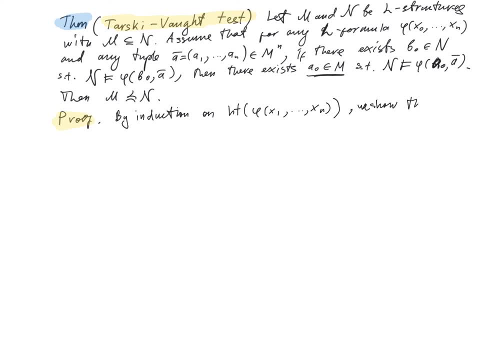 We will show that for any tuple a bar from the smaller structure m, we have that m satisfies phi of a bar if, and only if, n satisfies phi of a bar, which is exactly the condition required for been an elementary substructure. First, the case of height 0, when the formula phi is atomic. 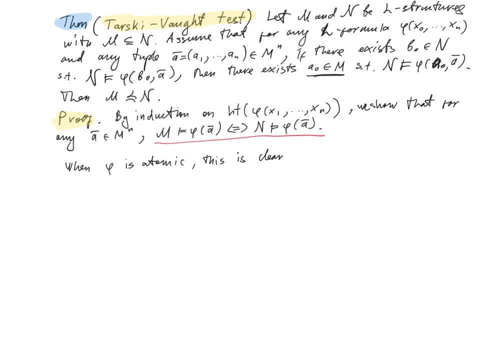 This is kind of interesting. since M is a substructure of N, by assumption, the case of logical connectives is also clear. so what remains is the case when Phi of X1 through XN- is the formula equal to the formula exists: X0, Psi of X0, X1. 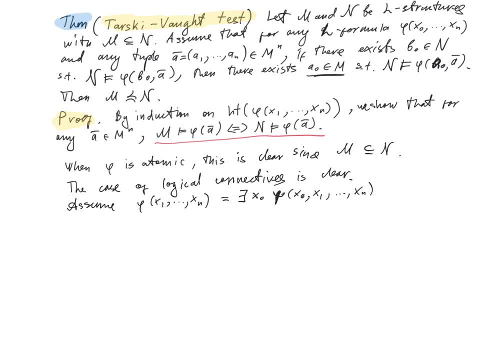 through XN for some Psi with height Psi strictly less than the height of the formula Phi. Also, note that as the variable X0 is not free in the formula Phi, we may assume that X0 is different from all the variables. Xi for i from 1 to N. Now let a bar be a tuple a1 through an from M, then we have 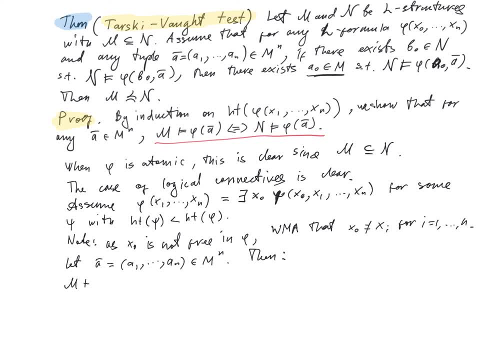 the following equivalences: The structure M satisfies Phi on a bar if, and only if, by the definition of satisfaction there exists some element a0 in M, such that M satisfies Psi of a0. a bar psi is a formula of smaller height by the inductive hypothesis we have that this is: 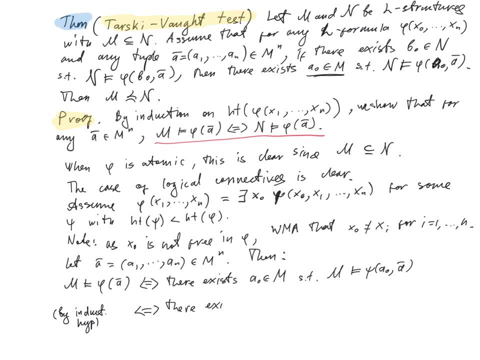 equivalent to: there exists a0 in M, such that N satisfies psi of a0 a bar. In turn, this is equivalent, by the assumption of the theorem, to saying that there exists some element b0 in N, such that the structure N satisfies psi of b0 a bar. 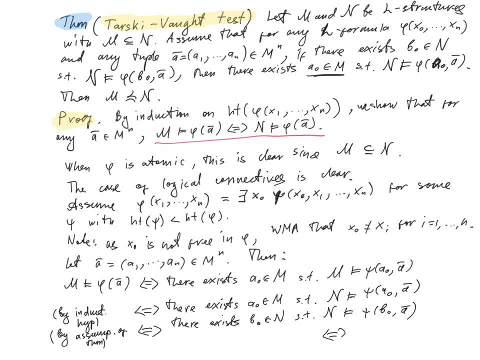 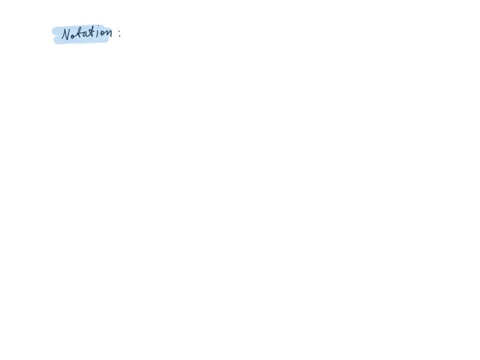 Okay, Which of course is equivalent to N satisfies. exists x0 psi of a bar or, equivalently, N satisfies, phi of a bar. This concludes the inductive step and hence shows that M is an elementary substructure of N. Notation: 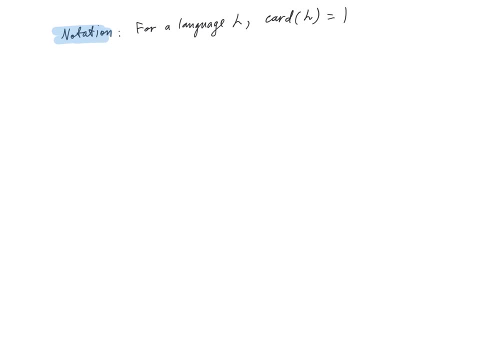 Given a language, l, we will write the cardinality of l, which we may also write alternatively as: the cardinality of l, using the usual symbol of cardinality is simply the cardinality of the set of all the bigger parts of a box. 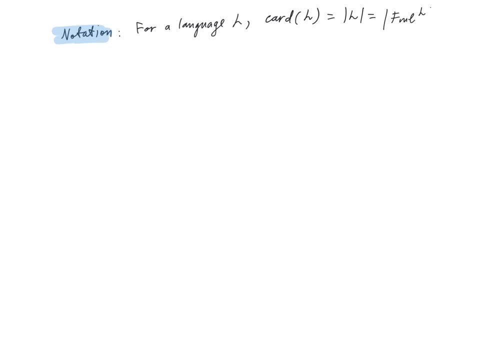 Okay, This is exactly for this. This is exactly how we evaluate, look, meaning this beautiful, very, very beautiful language. It must have all of these boboth, of course, not common demolition, but a totally different L formulas. So the first two are, by definition, the latter one the. 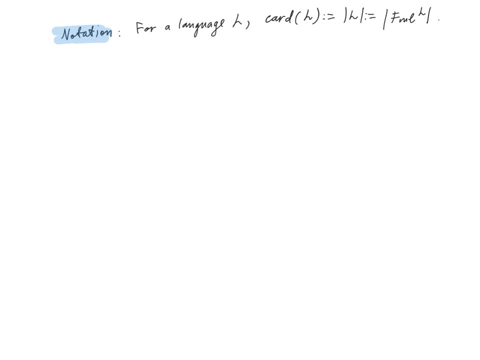 cardinality of the set of formulas. Now note that the cardinality of L is greater or equal than the cardinality of the set of terms of L, and of course, this is always greater or equal than aleph-node, so this is always infinite. 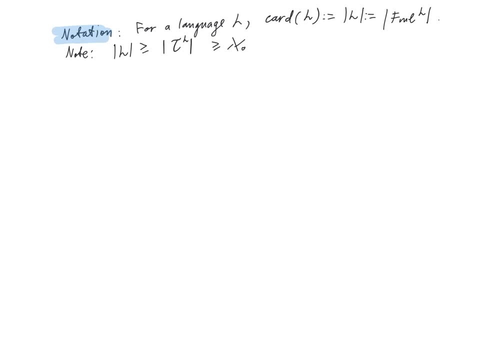 even if the number of non-logical symbols in the original language was finite. Now we can use the Tarski-Watt test to prove the following fundamental theorem, called the downwards Löwenheim Skolem theorem, which allows us to find elementary substructures of smaller cardinality. 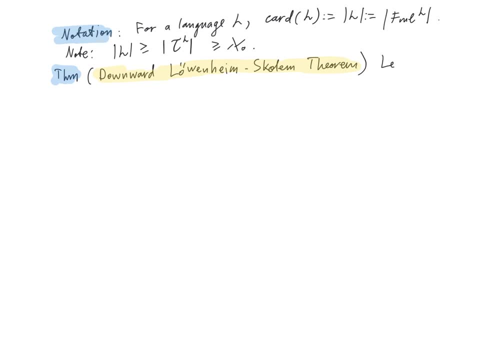 up to certain technical assumptions. So let M be an L structure and let A be a subset of the base set of M. assume also that the cardinality of M is greater or equal than the cardinality of the language L. then there exists: 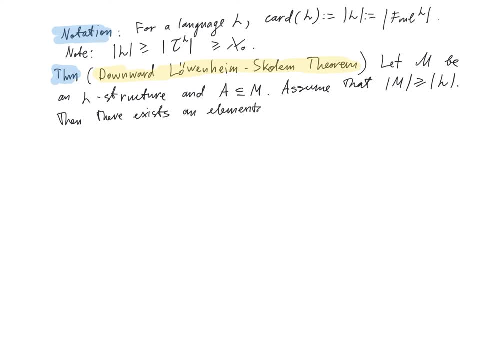 an elementary substructure M0 of M, such that the base set of this substructure contains this set A that we were given and such that the cardinality of this substructure is given by the maximum of the cardinalities of the set A and the cardinality of the language. 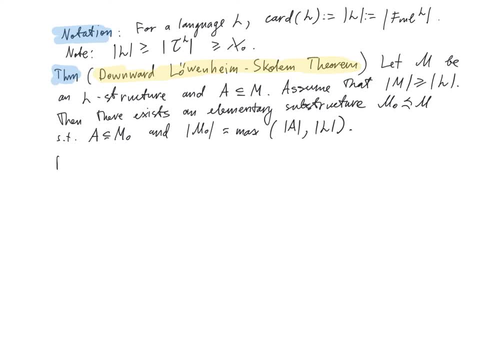 Proof. First, note that, enlarging the subset A if necessary, we may assume that the cardinality of this subset A is greater or equal to M than the cardinality of the language. so, of course, note that since we're only aiming to find an elementary substructure containing A of size, the 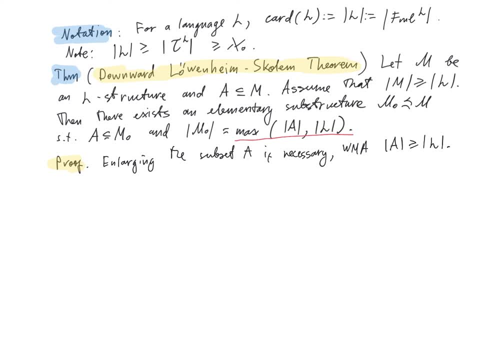 maximum of A and L. if we add some more elements to A, but at most L many we can. we do not change the conclusion if we can prove the theorem in that case. so we may assume then without loss of generality that A has cardinality at. 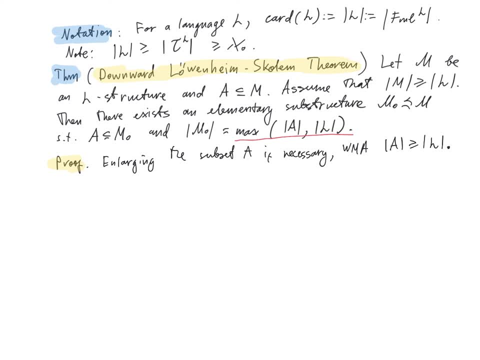 least the cardinality of the language. now, in this proof, when we have an unempty set B, a subset of M, we will denote by B tilde subset of M the base set of the substructure generated by the set B, so by which we mean B, M. 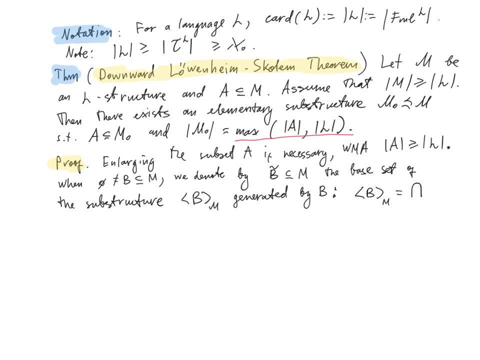 is the intersection of all substructures M' such that M' is a substructure of M containing B. note that the intersection of two substructures of M containing B is again a substructure of M containing B. hence this intersection is itself a substructure of M. 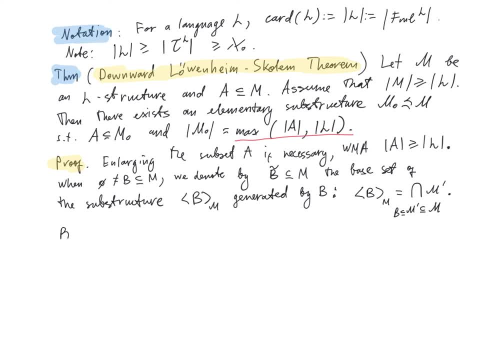 and we can write B tilde the base set of this substructure as the set of all elements of the form T interpreted in M, evaluated on B1 through Bn, where T is a term with the free variables X1 through Xn, the language L and b1 through bn are some elements of the set B. So this: 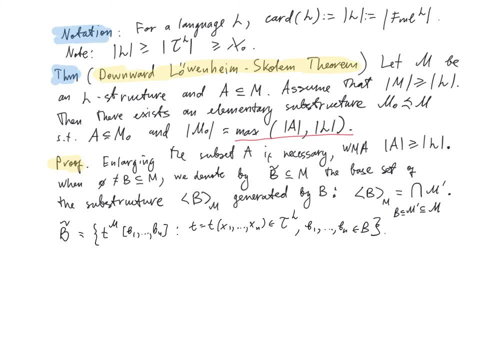 gives us an expression, a presentation for the base set of the smallest structure containing B, since it has to be closed under terms and we see that all the elements are of this form. In particular, we have that if the cardinality of B is greater or equal than the cardinality of the language L, 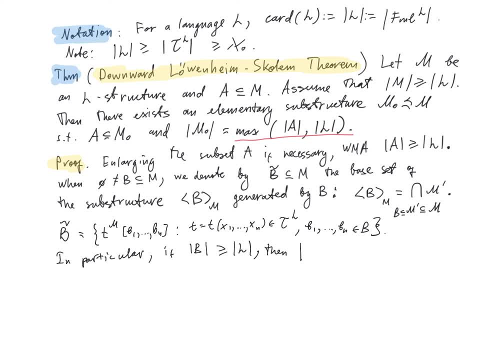 then the cardinality of the set B is equal to the cardinality of the set B tilde, since there exists a surjection from the set of all terms times the set of all finite tuples from the set B onto B tilde. So this is of course because of this presentation for the 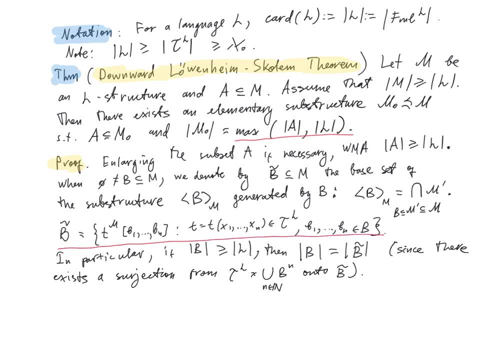 base set. We see that every element is given by picking some finite tuple of elements from B, for some n, and by a term applied to it. so then the set of all such pairs term-tuple from B subject onto B tilde. So of course this. 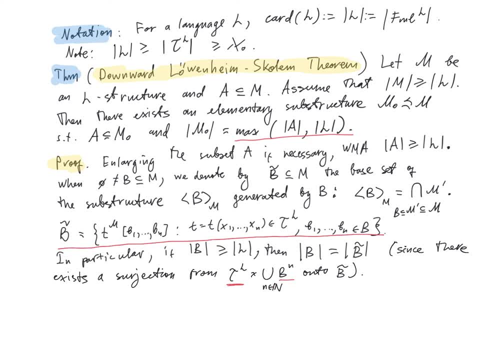 gives into a higher component, us the cardinality bound, because the cardinality of the number of terms is at most L, but, as we remarked earlier, and the cardinality of the set of all finite tuples from B is just the cardinality of B, assuming that B is infinite. so less, or 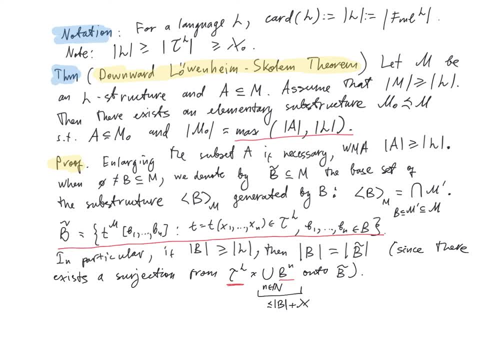 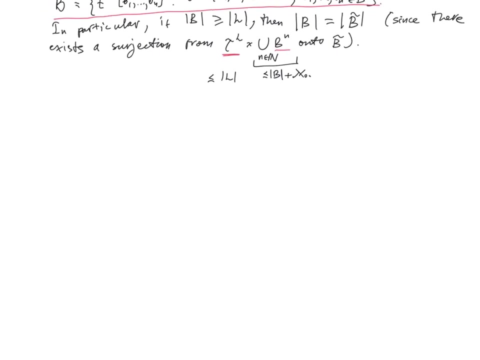 equal than B plus Aleph node, and so less or equal than L. so all together we get that the cardinality of the base set of a structure generated by B, B tilde, is equal to the cardinality of the set B itself We are going to define. 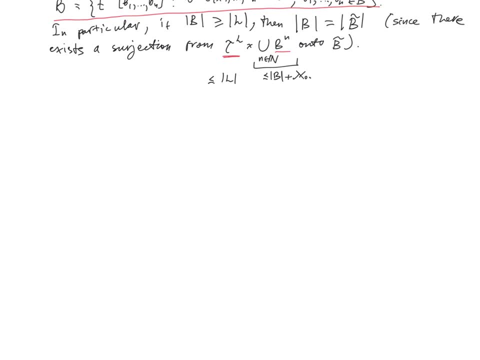 inductively a substructure containing the set A and B. A that we are given so that it is going to be closed under existential witnesses, as required by the Tarski-Watt test. Towards this purpose, we first let A0 be the substructure of M generated by the set B that we are starting with, and we 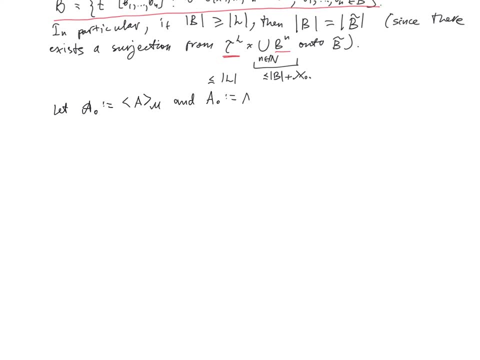 let A0 be the base set of this substructure generated by A. This is the base step of the induction. Now, assuming that AI is a subset of M which is already defined, we define the set AI plus one as follows: Now we could have: 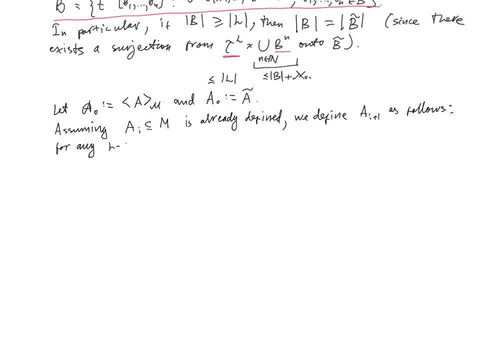 an KY di chapter for this. that's apply in for any L-formula Phi of X0 through Xn and any n-tuple xn, a bar of elements of the set AI, If we have that M is zero, or a bar of M against xn. and since the elements of M are zero, there is no Built-in expression for the set A To which we can say that the set AI, which is a subset of a set aside from an affogreat. Yes, exactly now that you've known that the sets A and B are misaligned. 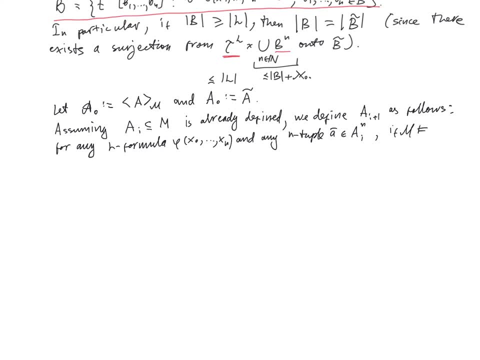 so we must now try to continue that If we have that M, that B is infinite, then we can randomize this set for a set A and B with this set is because the set B is infinite satisfies phi of b0, a bar for some b0 in M. so anywhere in the base set of the whole structure M. 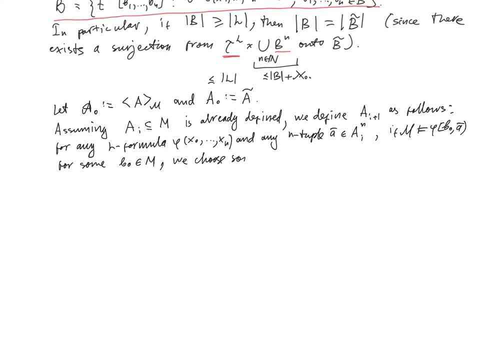 then we choose some element c which we denote as c of phi a bar, since it depends on the formula and on the tuple in M, such that M satisfies phi of c, of phi a bar a bar. So any b0 witnessing the satisfaction, we pick one and we denote it as c of phi a bar. 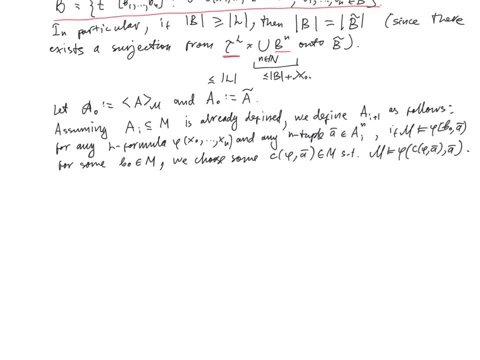 So note that there could be many different b0s which satisfy phi b0 a, but we just pick one and then we set b? i plus 1. To be the set consisting of a- i, together with the set of all elements of the form c, phi, a bar. 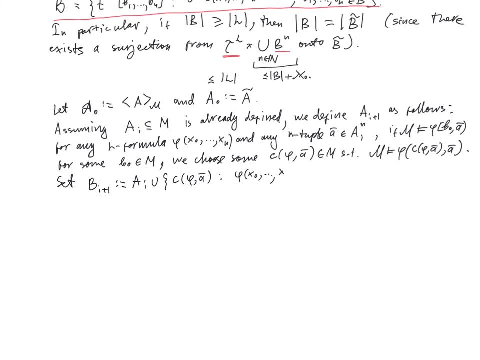 for phi of x0 through xn, a formula in the language L, and a bar, a tuple from a i of length M And finally, we let a? i plus 1 to be the base set of the structure generated by the set b i plus 1,. 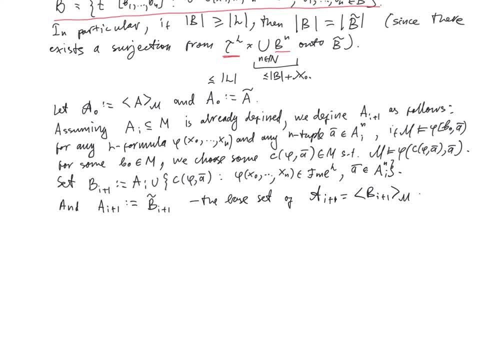 which we denote as the substructure of M, a curly, a, i plus 1, and i plus 1.. This gives us the inductive definition of the sets: a, i for all natural numbers, i, and then we let M0 be the union of all the sets. 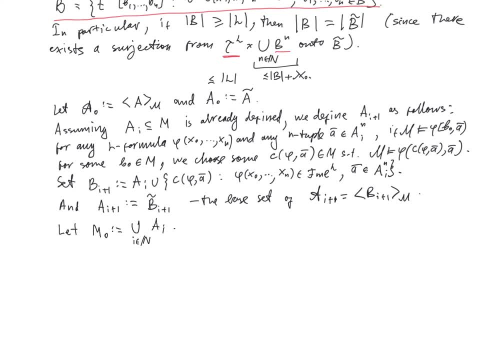 the union of all the a i's. then we have that the set M0 is non-empkey because, recall, we're assuming that a has quality, cardinality, at least a language. so it is in particular non-empty and is contained. 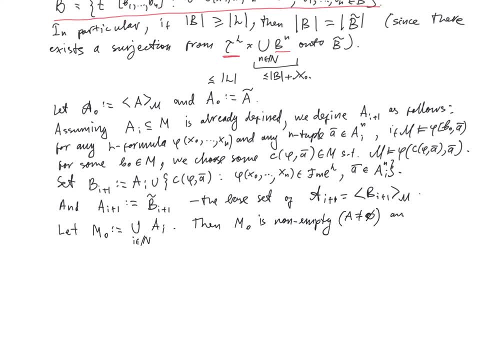 in M0. And also M0 contains C, M. the interpretation of the constant symbol in M for any C, a constant symbol of L, and M0 is closed under the functions given by the interpretations of the function symbols In M for any F, a function symbol of the language L. hence we have that M0 is the base. 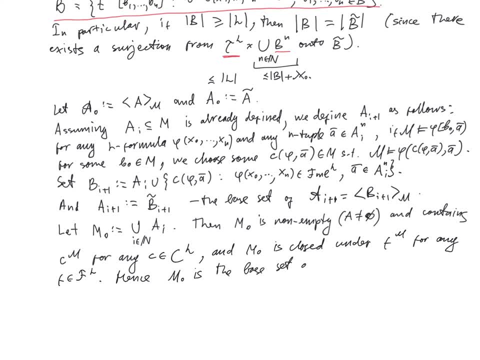 set. So M0 is the base set of a substructure, which we will denote as M0, of the structure M. So a union of the base sets of substructures is itself a substructure. Now we are going to apply the Tersky-Watt test to show that M0 is, moreover, an elementary substructure of M. So we are going to apply the Tersky-Watt test to show that M0 is, moreover, an elementary substructure of M. So we are going to apply the Tersky-Watt test to show that M0 is, moreover, an elementary substructure of M. 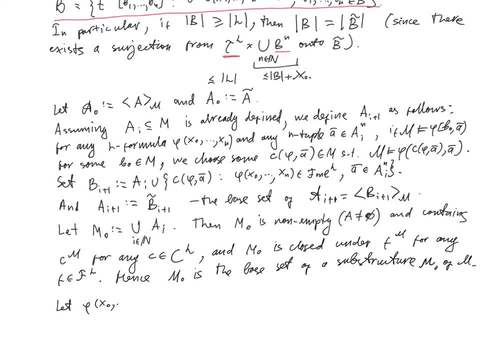 Towards this purpose. let phi of x0 through xn be an L-formula, a bar, a tuple from M0 of length n, and B0 is an element of the whole structure M, such that M satisfies phi of B0. So we are going to apply the Tersky-Watt test to show that M0 is, moreover, an elementary. 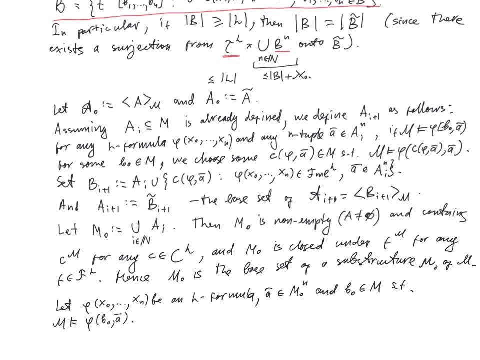 substructure of M, such that the Tersky-Watt set of M is, moreover, an elementary substructure of M. Then we know that there exists some natural number, capital N, Such that these elements of the tuple A-bar, which we denote as A1.